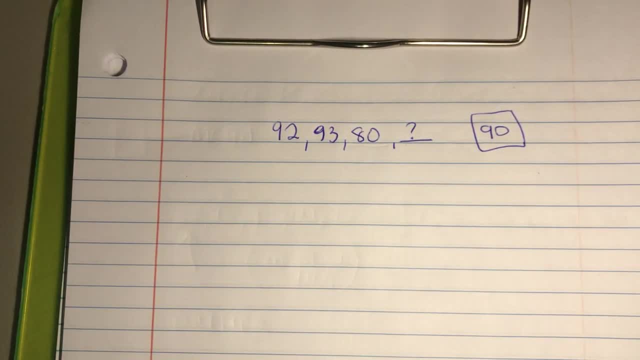 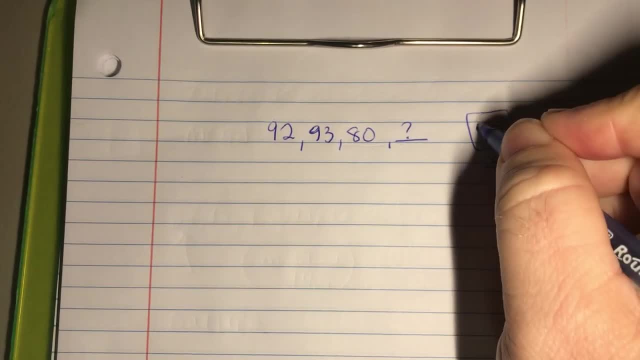 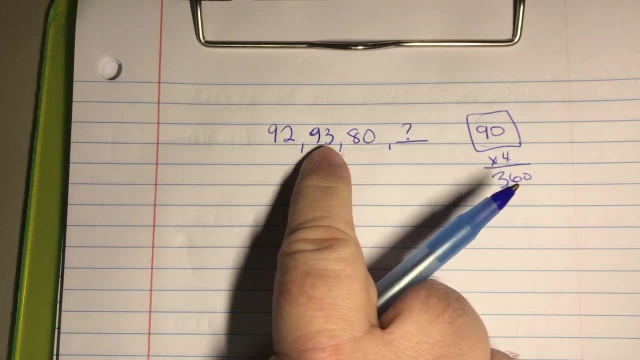 I know that for all four tests I need to have the total of what four times 90 would be. So four times 90 is well 360.. So I know that these four numbers need to add up to this in order for me to divide this by four, to go back to 90. 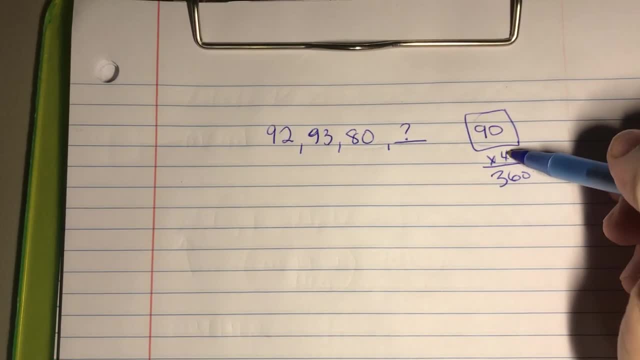 right Makes sense. I mean, I mean there's four tests. I want the average to be 90. Well, the average is when you take the total and divide it by whatever the number of tests are or the number of data, to get your average. So we're kind. 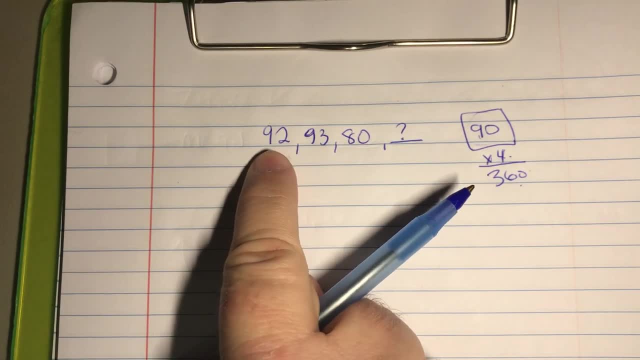 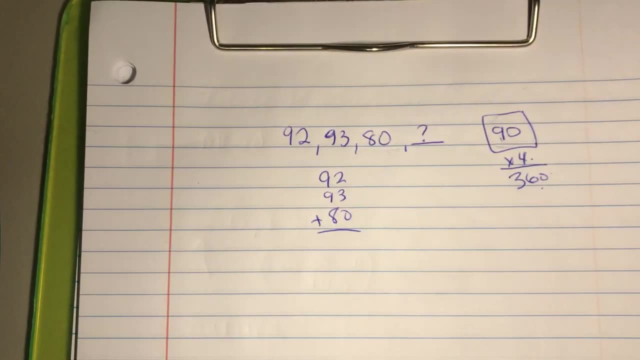 of working backwards here. So let's take these other numbers that we actually know. Let's take those and add them, So we have 92 plus 93 plus 80. Now, remember we're working with data and we have a lot more numbers than the ones you'll be doing. 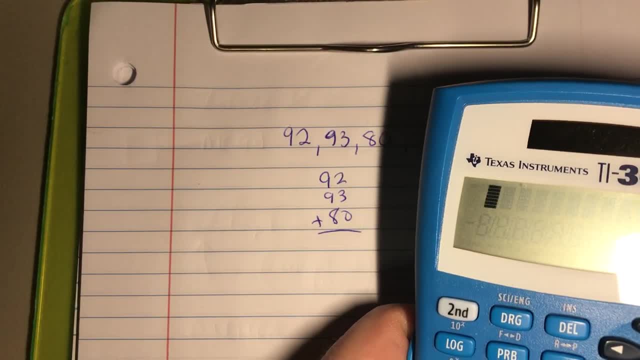 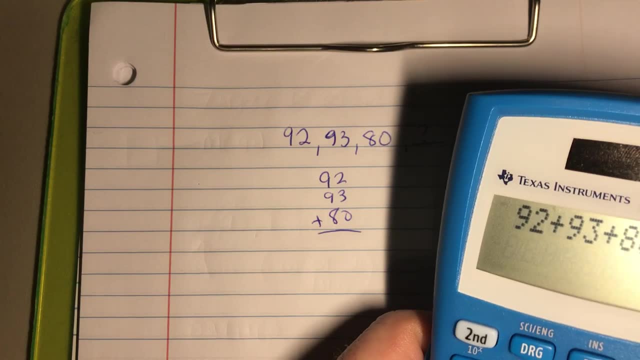 today, So grab that calculator. It's okay, We're going to take 92.. I know we can do this without a calculator, but there's going to be a lot bigger numbers today, So get that ready. So if you put the numbers incorrectly, you have 92 plus 93 plus 80 is equal to. 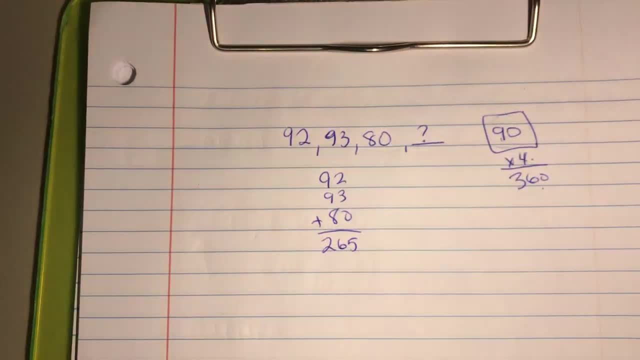 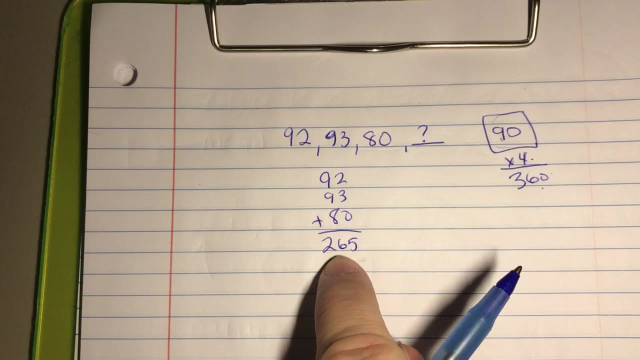 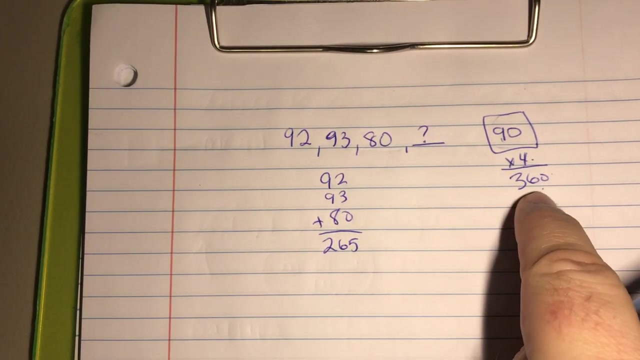 265.. right, So I want to find the missing number. Well, if all of these equal 265 and I need one more number to get that, what are you gonna do? You know that all of this added together will get you this, because this, divided by this gets you this. Well, of course, we're going to just 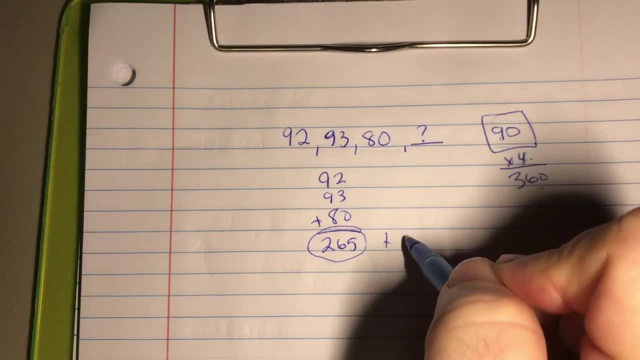 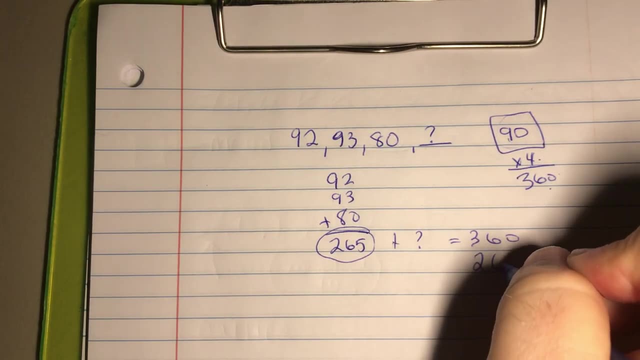 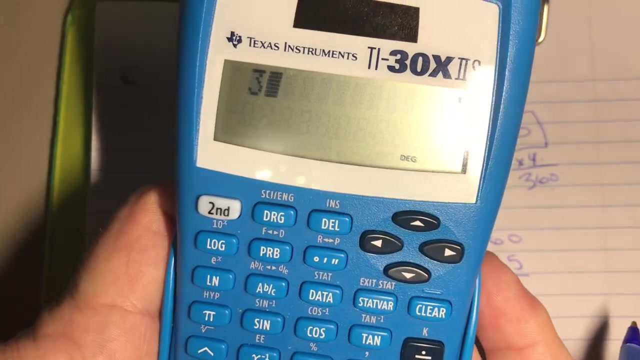 take this number and we're going to add it to the number we don't know to get this one. I mean, obviously, if we don't know that number, we just subtract this from this, we just subtract this from this. all right, so we grab our calculators and we put 360, we're subtracting 265.